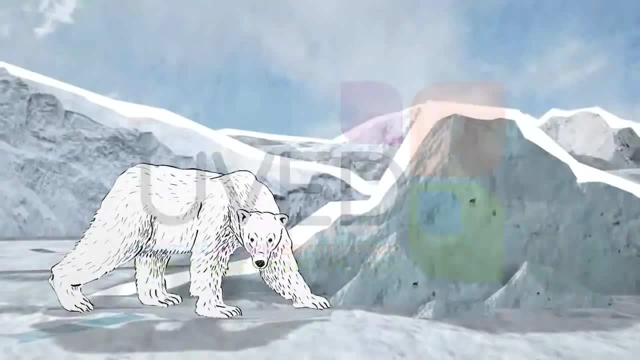 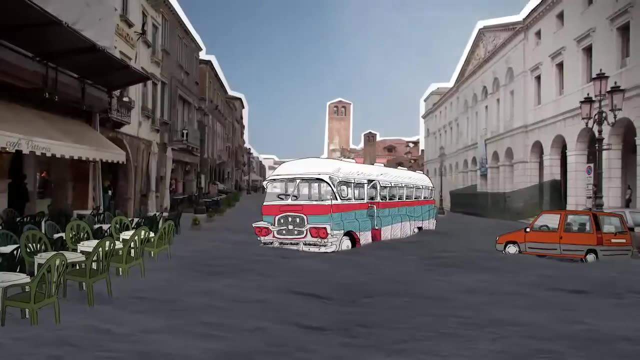 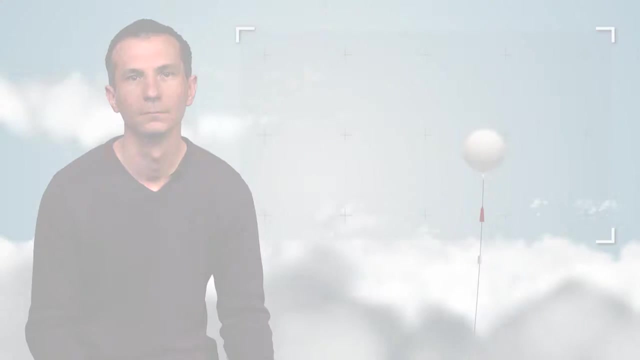 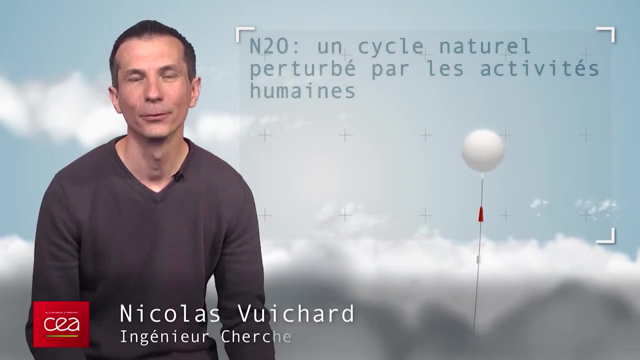 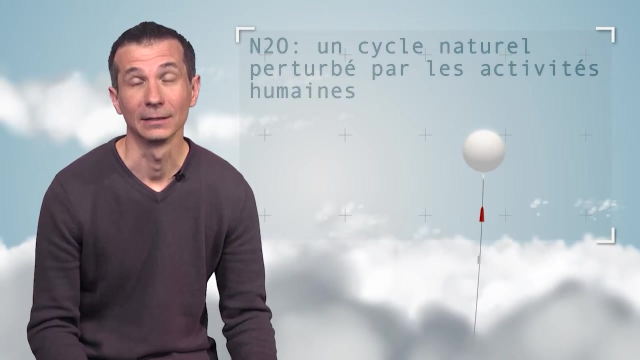 In this video, I'm going to tell you about N2O emissions and the nitrogen cycle. like with other greenhouse effect gases, there is nitrous oxide, the concentration of which has increased a lot over the last 50 years due to human activity. 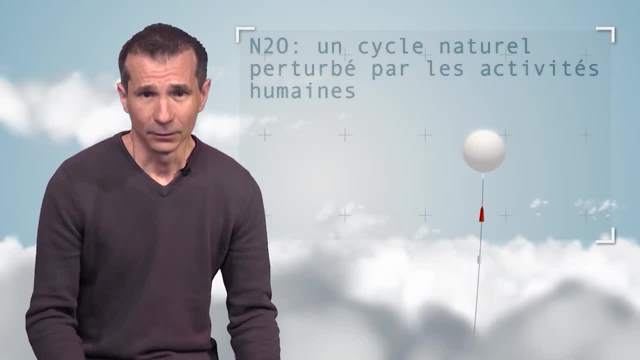 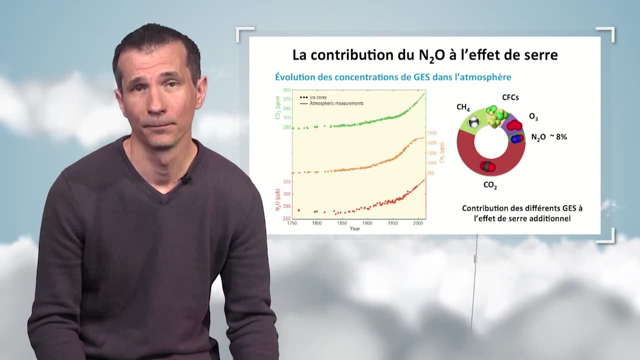 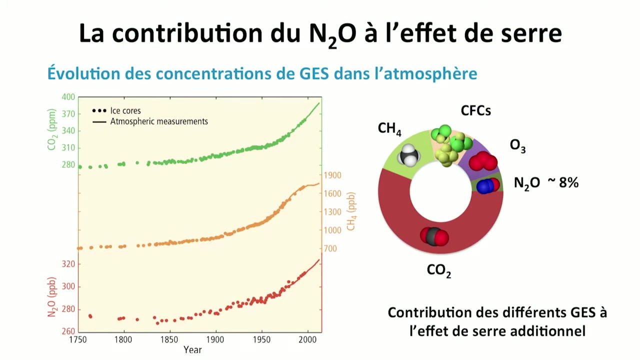 We estimate that the N2O concentration has increased and moved from 270 ppm in 1850 to more than 220 ppm nowadays. Now the concentration is 1,000 times lower than those. This is because of CO2, but because it has a strong warming capacity. the contribution: 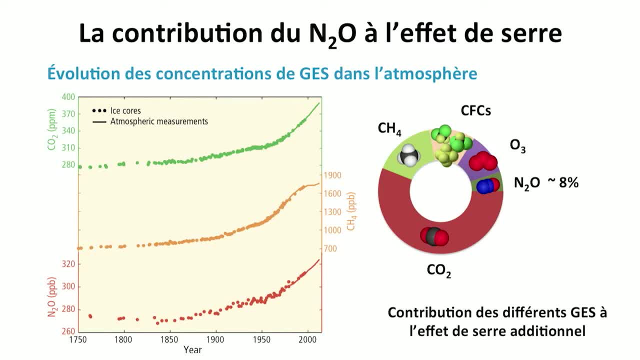 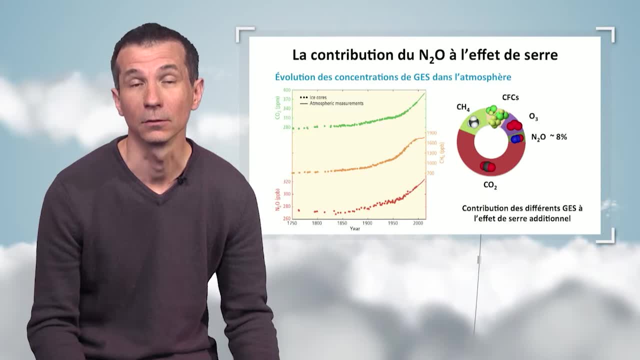 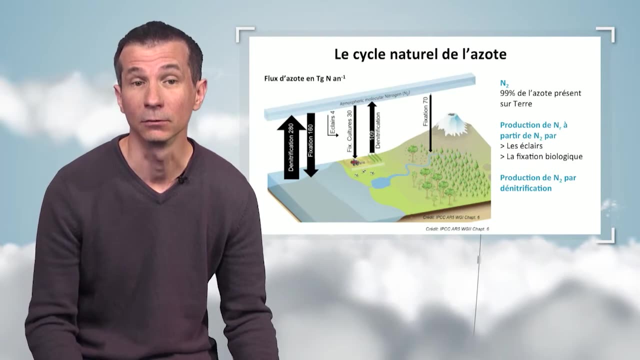 made by NTU to the greenhouse effect is still significant. We have reason to believe that N2O corresponds to 8% of the additional greenhouse effect ever since 1850.. In order to understand the concentration increase observed for N2O and related emissions, we 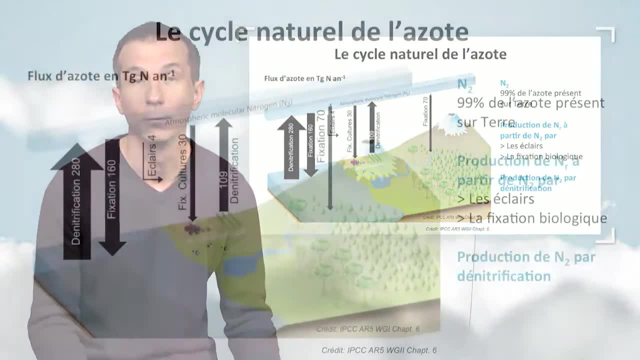 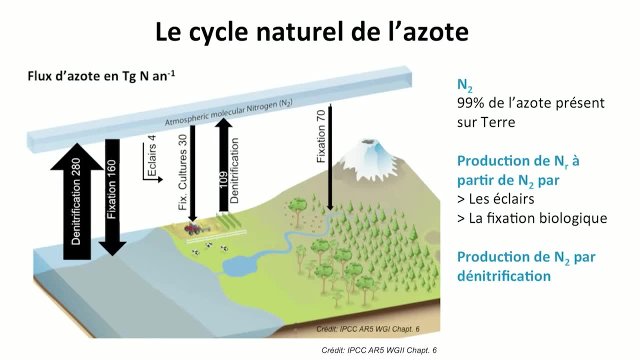 must look at the nitrogen cycle. The nitrogen constituent on Earth is N2O, made of two molecules of nitrogen. This is the main constituent in the atmosphere, but N2O reacts with no other constituent in the atmosphere. Therefore it's defined as inert. 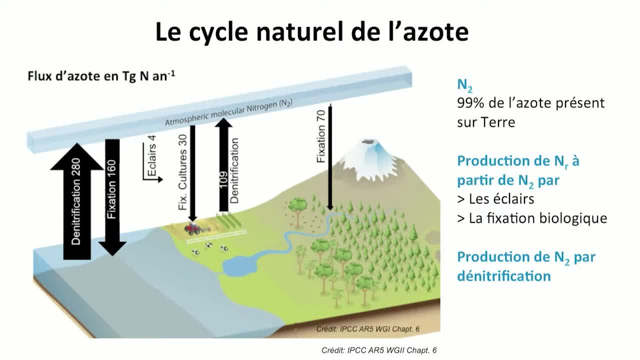 Before the industrial era, the two sources of nitrogen were nitrogen and nitrogen. This is the main constituent in the atmosphere, but N2O reacts with no other constituent in the atmosphere. The main constituent in the atmosphere, however, is nitrogen. The two sources which created the reactivity of nitrogen based on N2, were those combined. 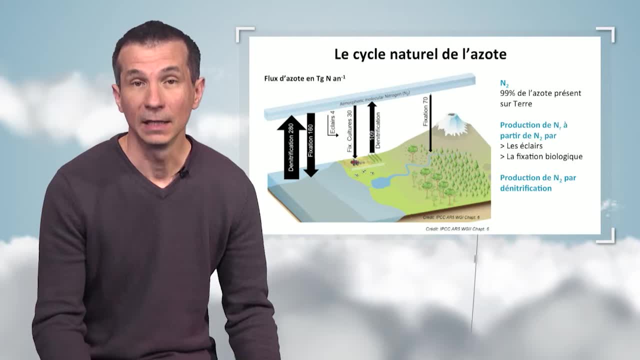 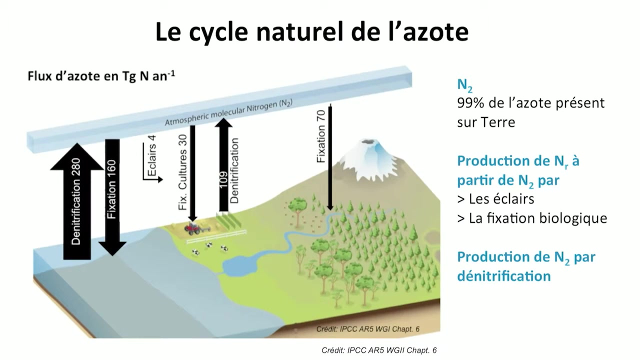 with flashes due to temperatures, leading to forms like NO or NO2.. More importantly, the second source was due to biological fixation of nitrogen. This was the second source created by local robots. This was an interesting observation. nitrogen- Natural nitrogen fixation is performed by bacteria in the ocean- cyanobacteria- and on 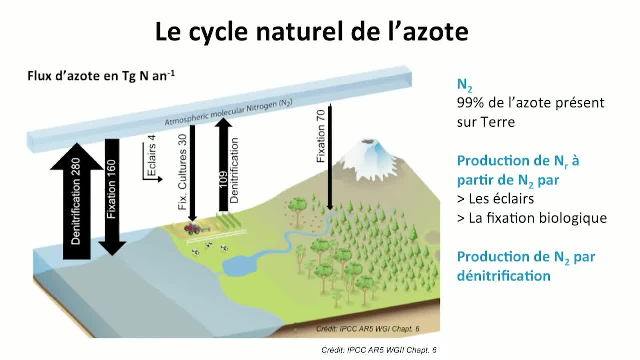 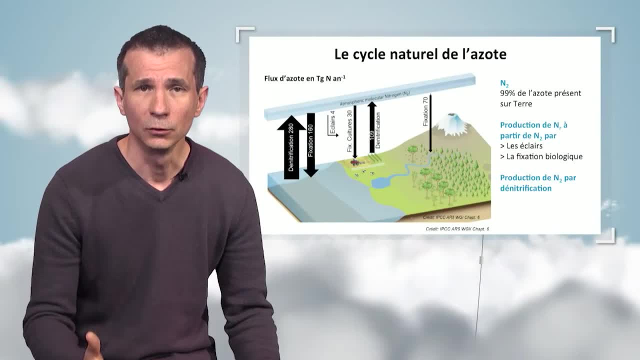 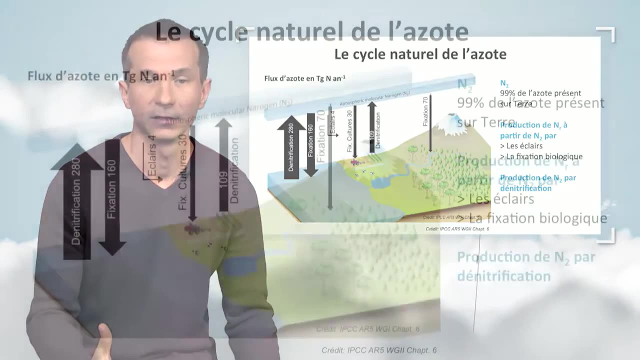 Earth rhizobia, which live in symbiosis with the root radicular system of pulses and leguminous plants. Now in the nitrogen cycle, we see the large arrow going from the Earth to the atmosphere. There is de-nitrification, an essential process in the nitrogen cycle, because it is the only one. 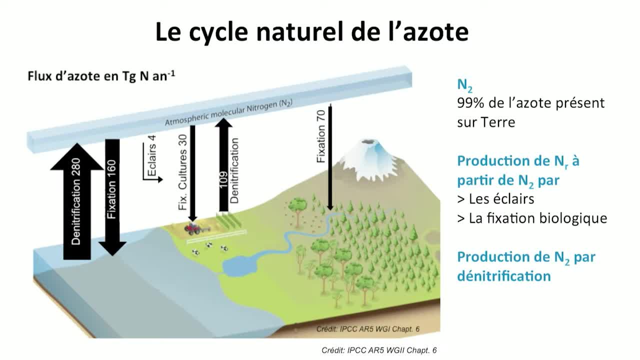 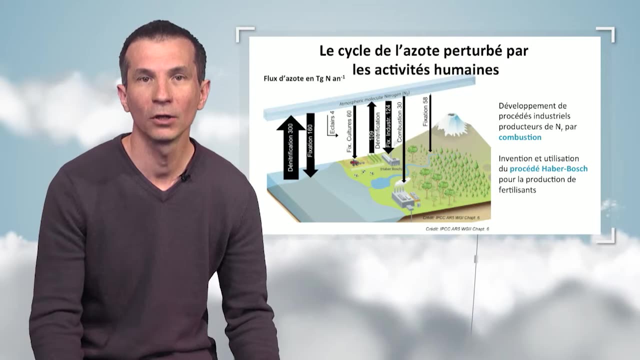 that allows for reactive nitrogen to come back to inert N2.. It plays an essential role in the nitrogen cycle because it closes the loop. It closes the cycle For more than a century. two more sources have added themselves to the historical. One is the use of the historical sources, combustion of fossil fuels due to industrial 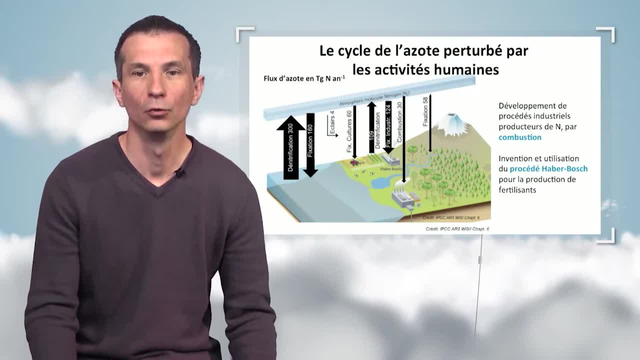 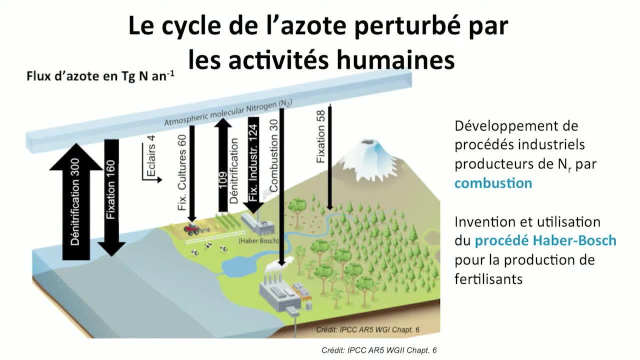 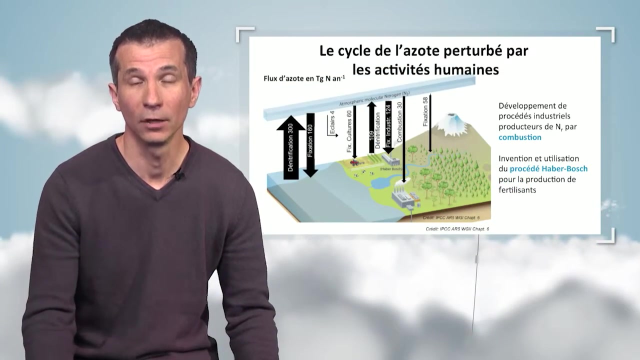 processes. And another source, the use of the Haber-Bosch process, which is a process to manufacture nitrogen-based fertilizers. This process was invented in the early 20th century and it is essential because a large part of the development of modern agriculture is based on. this process, And it is essential because a large part of the development of modern agriculture is based on this process. And it is essential because a large part of the development of modern agriculture is based on this process. And it is essential because a large part of the development of modern agriculture is based on the invention and the development of this process. However, this new source of reactive nitrogen has changed the nitrogen cycle. Annual sources of reactive nitrogen have increased by 150 telegrams of nitrogen ever since 1850, and entropic sources are equivalent to the natural sources with 150 telegrams of nitrogen. 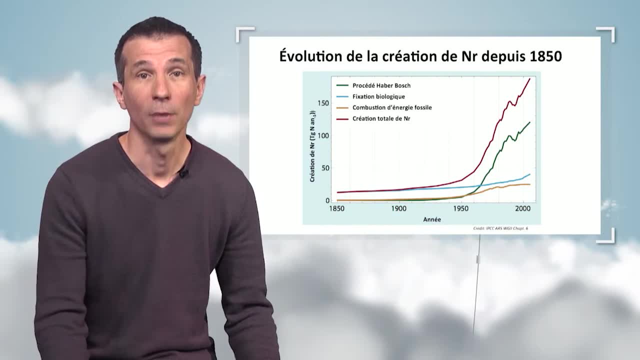 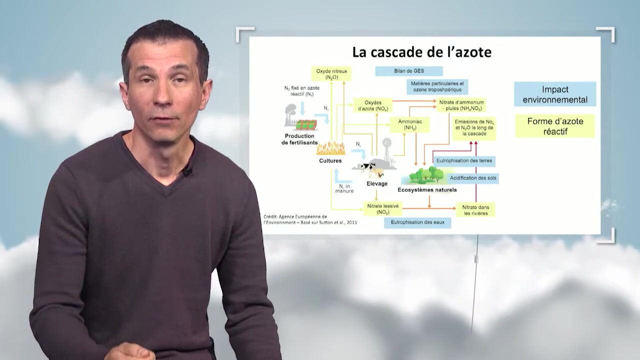 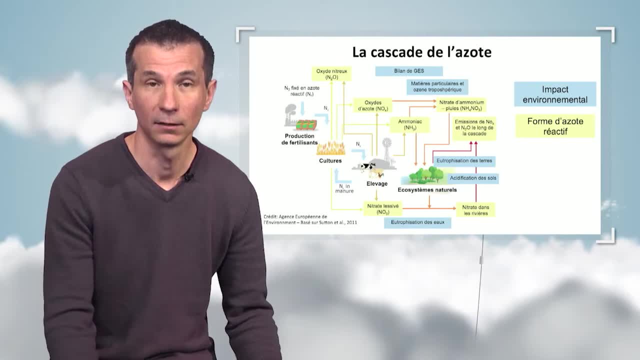 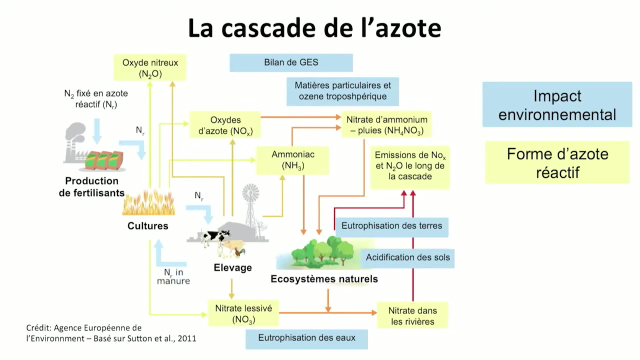 Sometimes there are leaks in the ecosystem, either directly from the plowed fields or indirectly. once nitrogen has been assimilated by the plants, and when the nitrogen is released During the circulation in the environment, nitrogen will be transformed, with a number of impacts on ecosystems, health and climate. 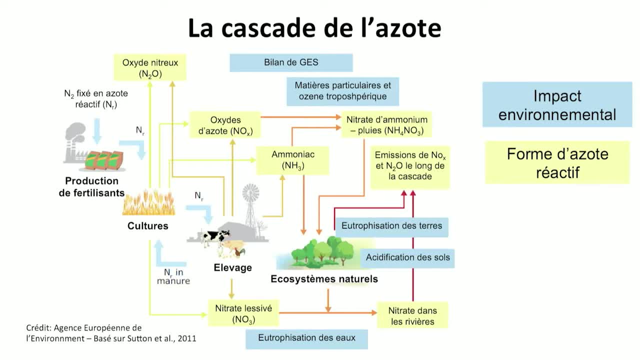 And this is the reason why we introduced a system called nitrogen cascade, considered as the sequential transfer of nitrogen within ecosystems and the consequences on the climatic impact. Here we see, for instance, in yellow ammonia nitrate and nitrogen oxide. 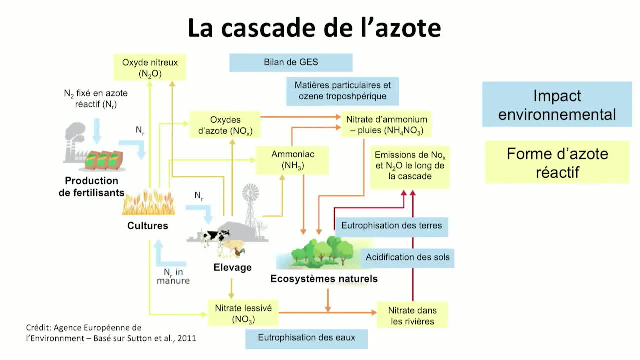 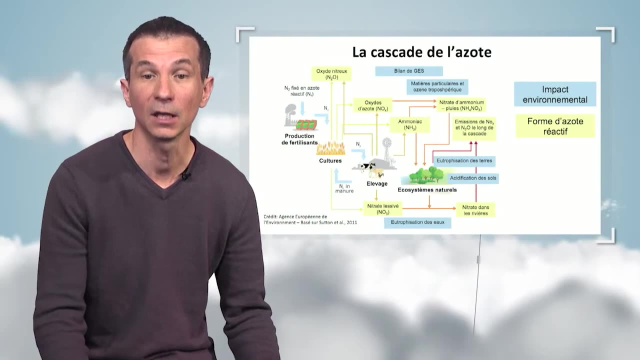 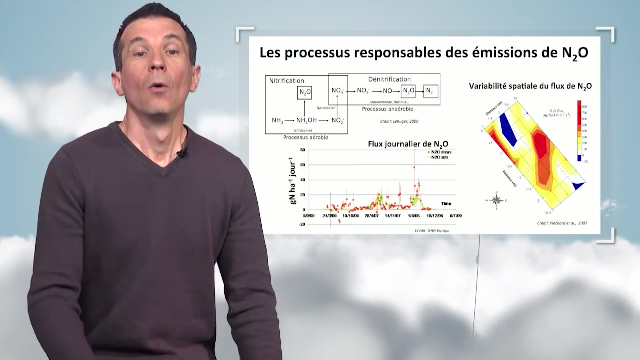 These emissions can then deposit themselves in the wet or dry form. Nitrates can accumulate in rivers and contribute to eutrophication of water. And finally, there is also nitrogen accumulated in the troposphere. Concentration peaks entail risks for human health and also. for ecosystem balances. Now, among the quantity of reactive nitrogen accumulated in the systems, we find also nitrous oxide, N2O. N2O is produced in the environment under two forms: nitrification and denitrification. Nitrification is a process that allows 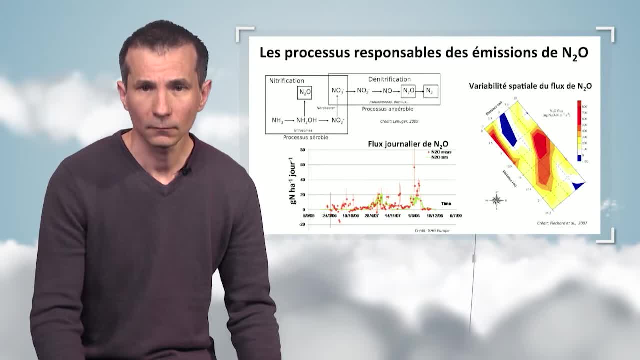 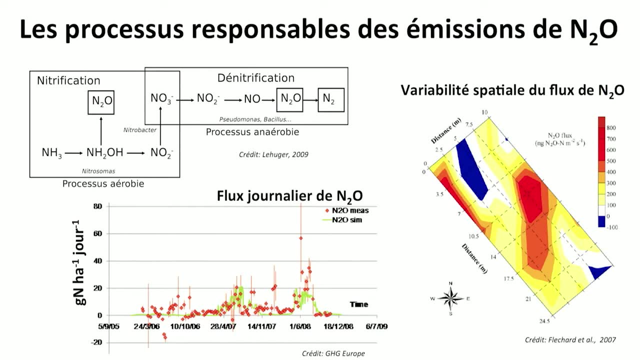 to produce N2 from nitrogen oxide. N2O, or nitrous oxide, is an intermediate product in the system. Nitrous oxide is also produced in the process of denitrifying kalkite, Nitrous oxide known to be the best nitrous oxide. 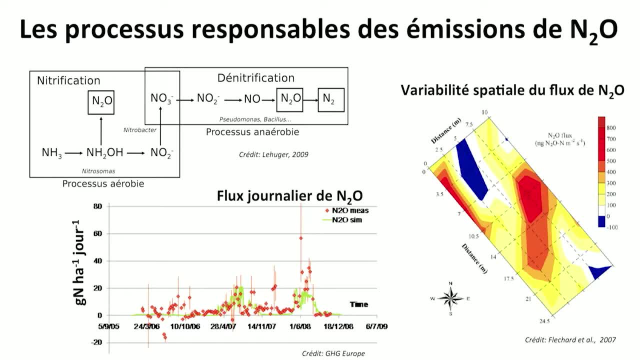 is then lie in the nitrification process. Then denitrification changes the ammonium into nitrate And we have seen that high concentrations of nitrate will lead to eutrophication of rivers. N2O is a co-product or a byproduct. 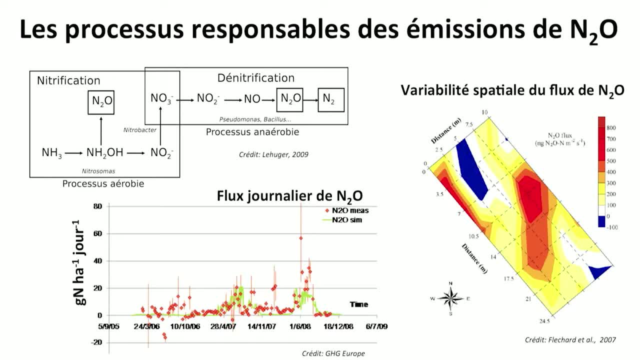 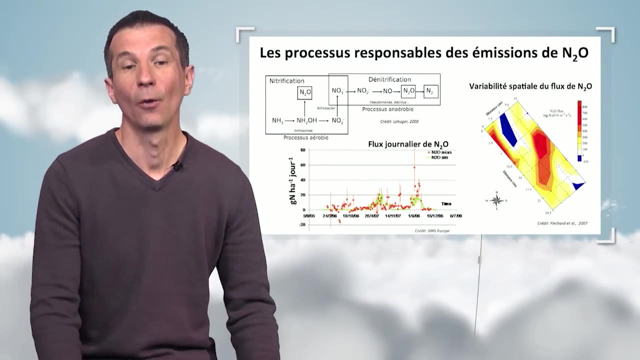 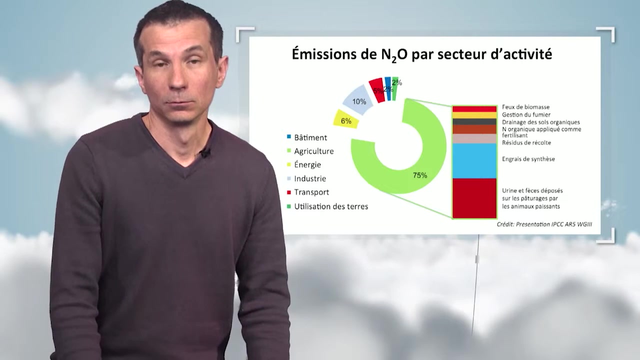 of the nitrification process shown in the two graphs: variability of N2O flows and spatial variability. time and space variability are very high. This is difficult to manage because we need to measure N2O released by fields and their use in the atmosphere, so there is a relative uncertainty regarding the flow of N2O. 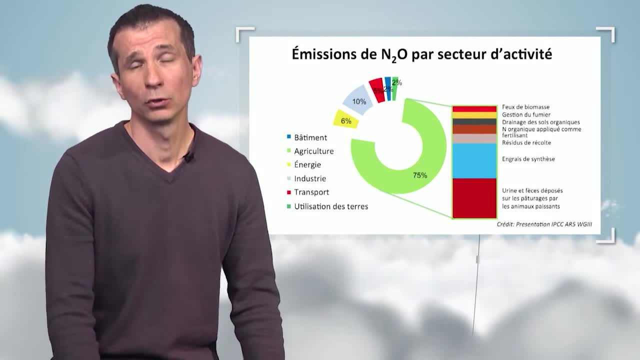 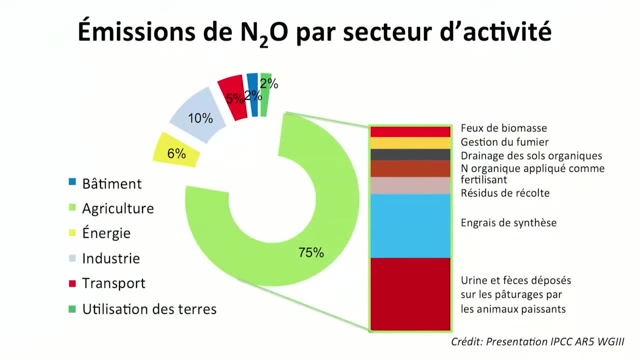 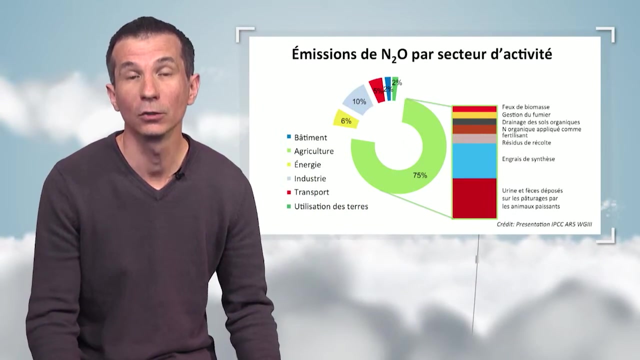 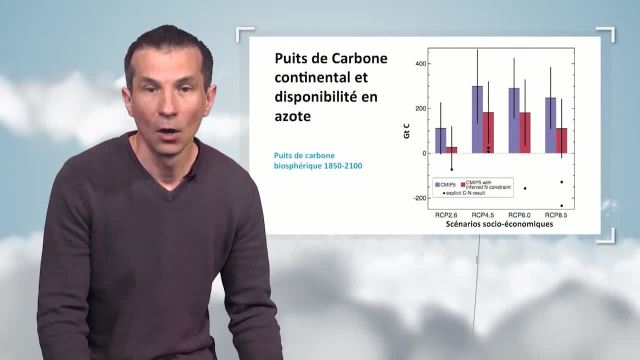 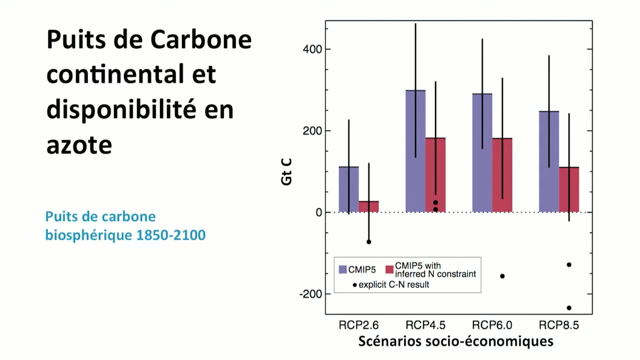 There are also cooling effects. Among the cooling effects, we can mention the presence of reactive nitrogen, which involuntarily fertilizes natural ecosystems. To this day, this phenomenon has maintained or even amplified the CO2's sink in the the terrestrial atmosphere, according to the last simulations, according to which this 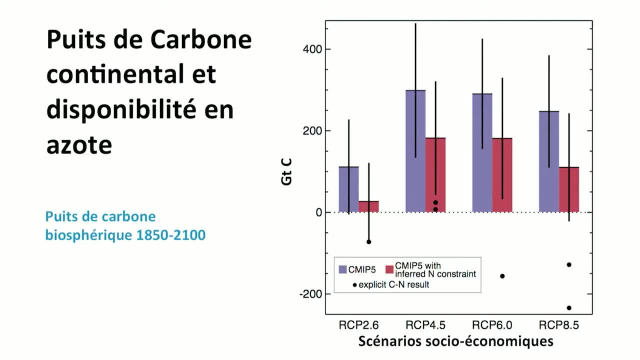 sink will be maintained in the next century because of fertilization happening with. N2O does not take into consideration the nitrogen cycle. Therefore, we have reasons to believe that the CO2 sink shown in blue could be decreased if the nitrogen cycle and the associated limitation of this nutrient were taken into consideration. 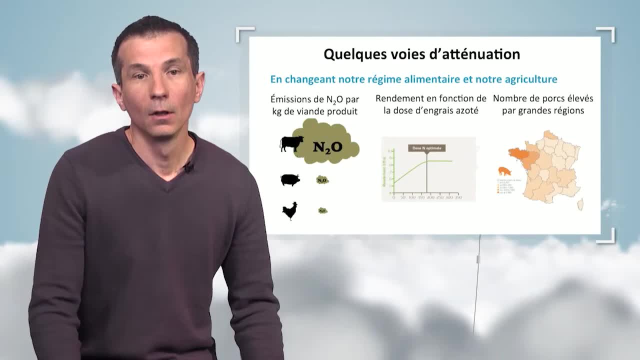 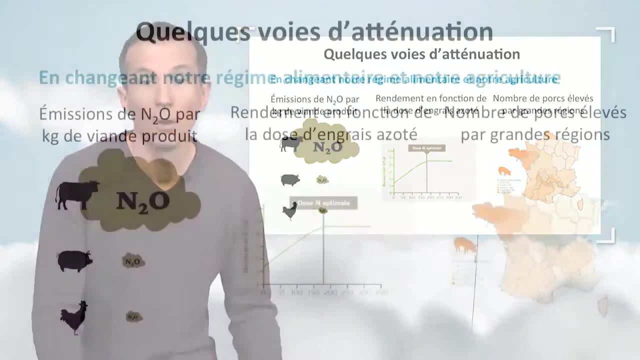 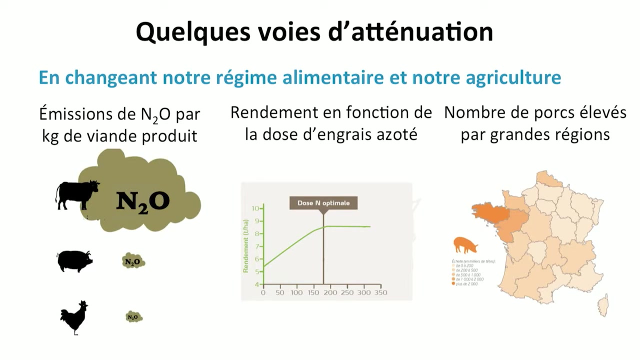 This is what is shown by the purple bars. In conclusion, although reactive nitrogen can have cooling effects on the climate, the detrimental effects of accumulation in the environment should make us think about ways to mitigate this phenomenon. For instance, we could We could do something about our eating habits, bearing in mind that pervine cattle breeding